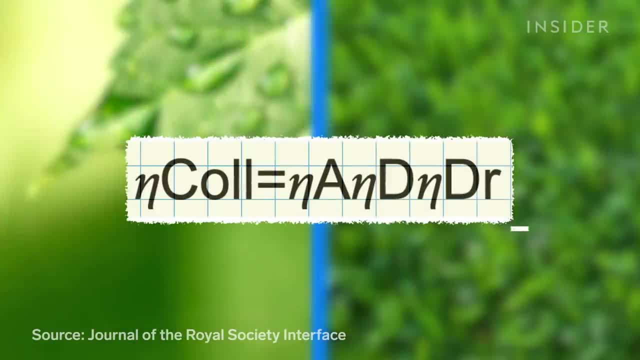 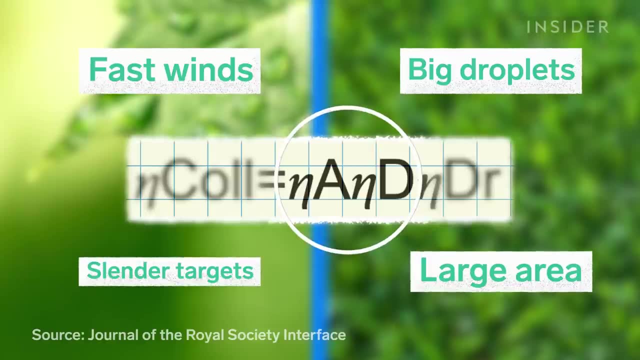 blades of grass, And their efficacy is determined by this complicated formula, Where these two basically confirm that fast winds, big droplets and slender targets across a large area are the best conditions for collecting, And this one represents the mesh's ability to drain the 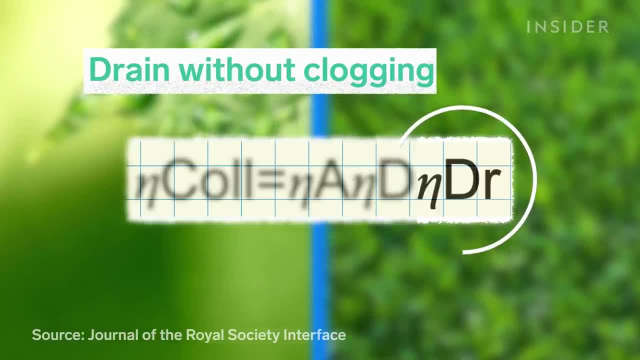 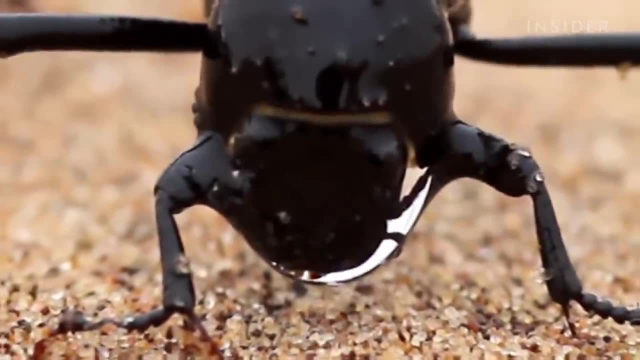 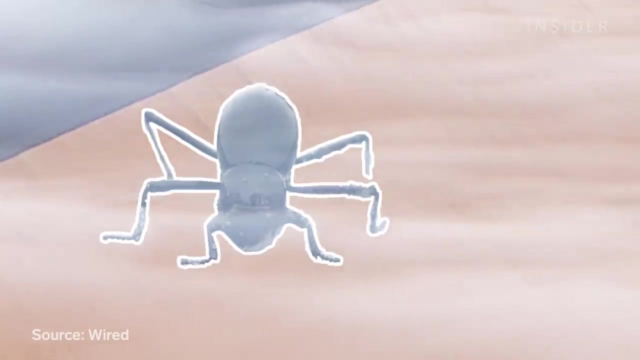 collected droplets into a reservoir without clogging. So, based on the formula, the Namib Desert Beetle shouldn't be able to do what it does, Since you know, beetles aren't made of mesh. And yet, when fog rolls in, the beetle climbs to the top of a dune and fog basks leaning down and into the wind Water. 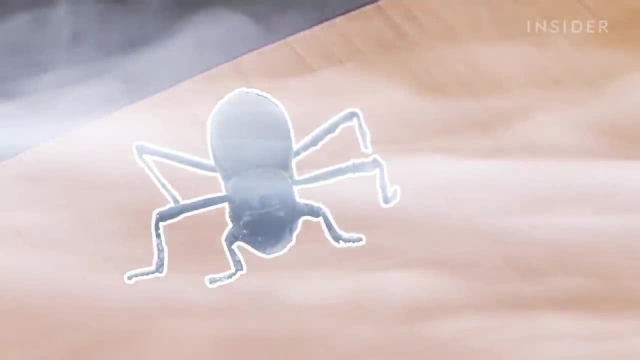 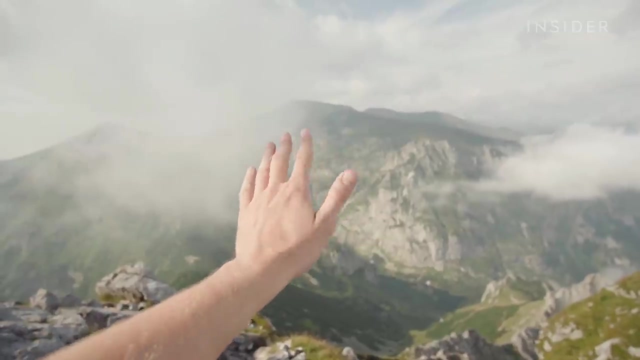 droplets collect on its back and roll down to its mouth. As simple as that sounds, it's very literally like trying to catch a cloud and pin it down. If you wave your fingers through mist, you don't see just where your fingers were and all the water collected. It just flows with the air right. 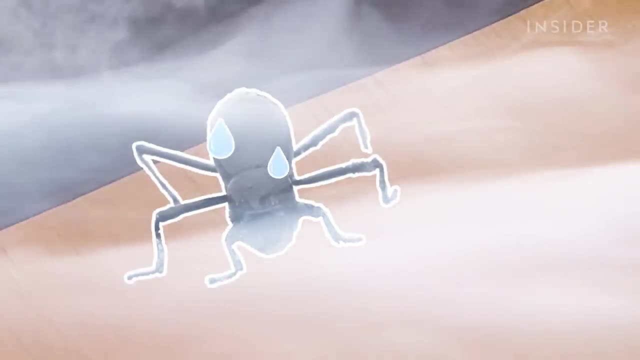 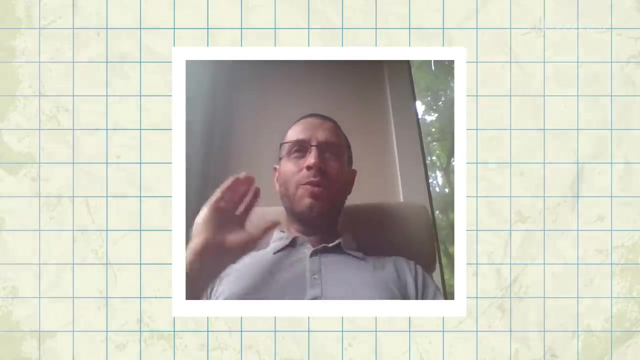 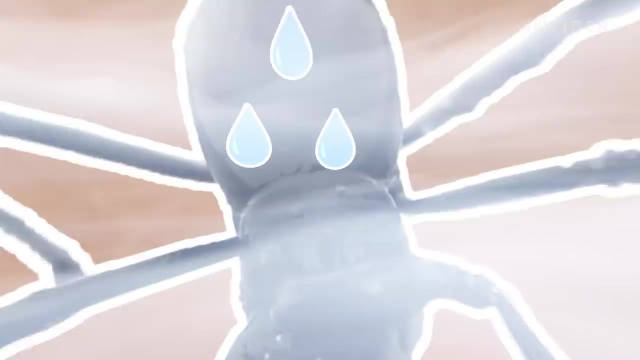 through them. But the beetle manages to do what we cannot. The secret is in its exoskeleton And it's very much a secret. We are far away from that still, Or we're getting closer. A lot of research has been done on how the water moves to the beetle's mouth, but almost none has covered how the 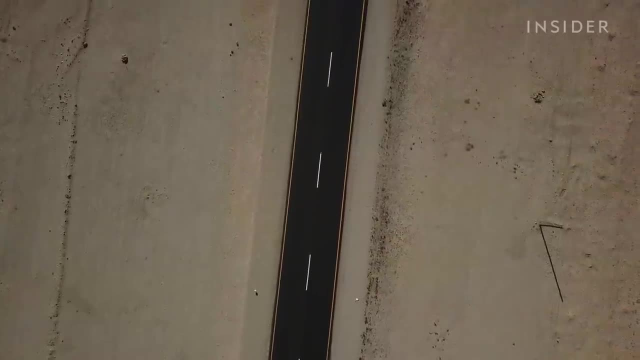 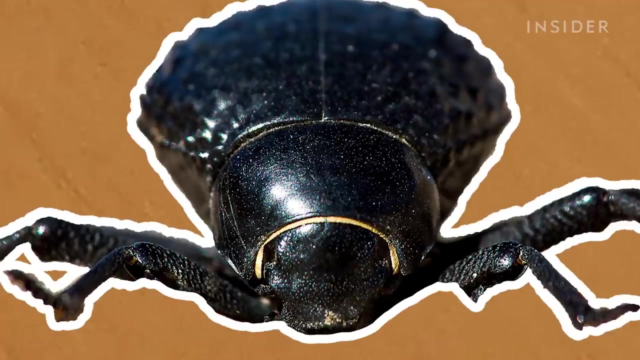 droplets get there in the first place? Hunter King and his team tried to find the answer, but hit an unexpected bump in the road. The original beetle that scientists started researching first had exactly that Bumps on its exoskeleton, And those bumps were theorized to have an impact on the 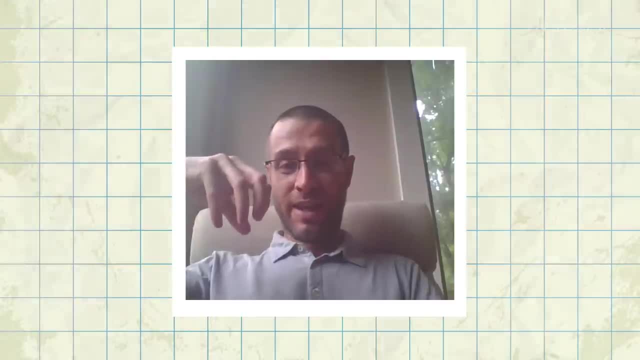 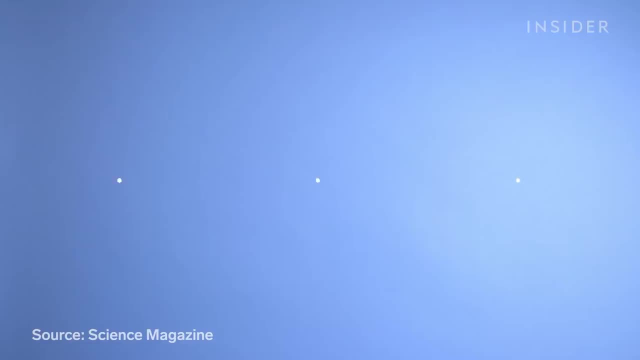 efficiency of fog collection. But It turns out the beetle that has the bumps is not one of the fog-basking beetles. King and his team decided to move forward with their experiment anyways. In the lab they 3D printed spheres and cylinders with various surface textures, Smooth ridged. 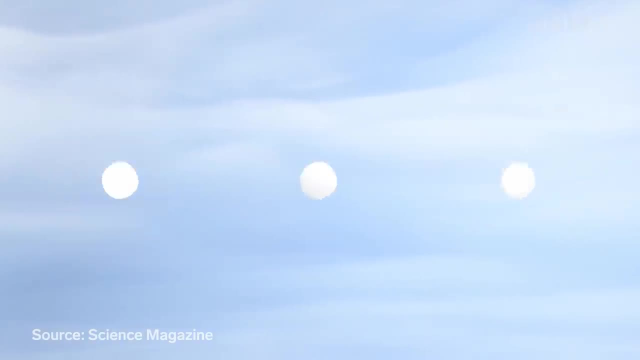 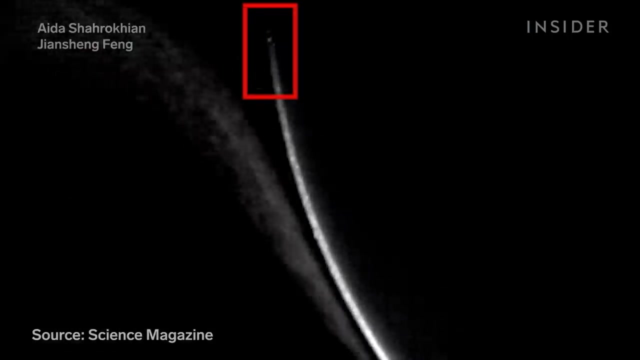 and bumpy. They then put the spheres in a foggy wind tunnel. Turns out the sphere with one millimeter bumps captured fog- two and a half times better than the smooth sphere If you add ridges that are maybe a little bit like the beetle that we found is the fog-basker. 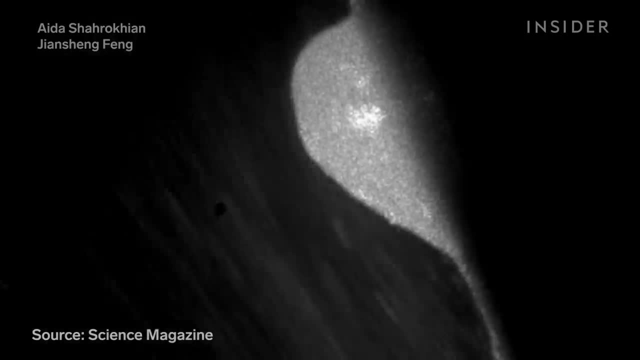 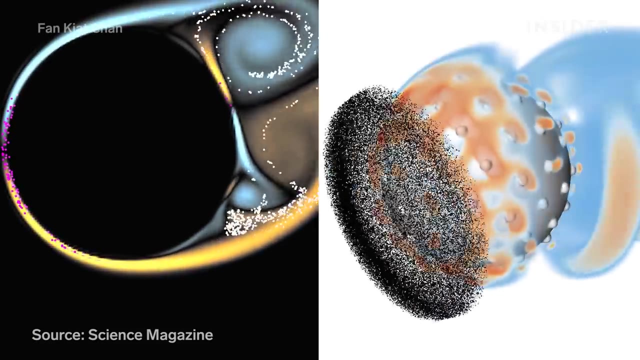 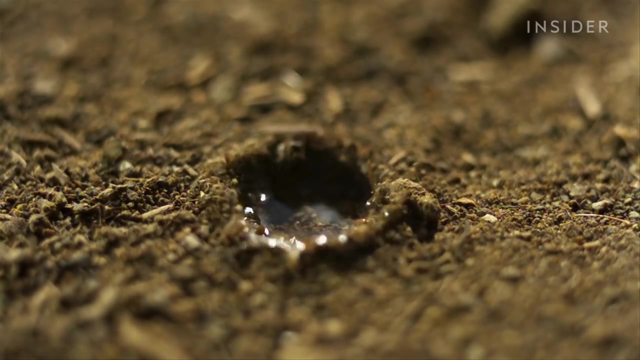 it's something like a factor of two, so it's still not small. Further research in partnership with computational fluid dynamics experts at the University of Illinois zoomed in even closer. They developed a computer model that tested droplets' ability to bump into a surface. Tiny water droplets have very little inertia and have to squeeze a film.